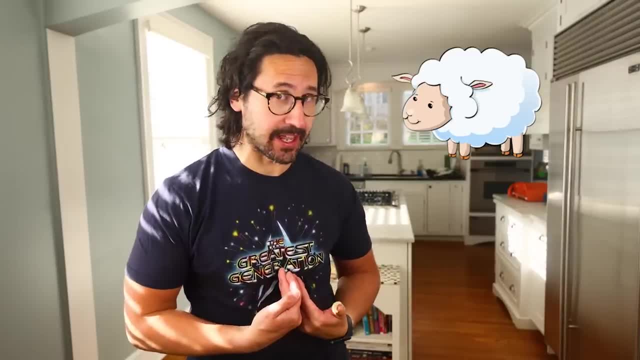 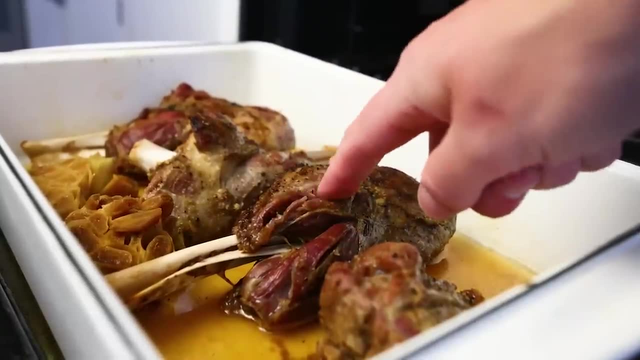 still want it. What are you saying? You saying I can't handle the Chilean stuff. Put them shanks on the scale, Meet me. But then I went home and spent several days cooking these shanks to develop a recipe you may have seen in my previous upload, And I was like, oh. 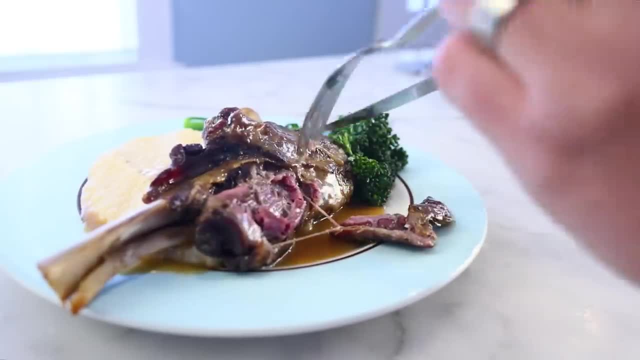 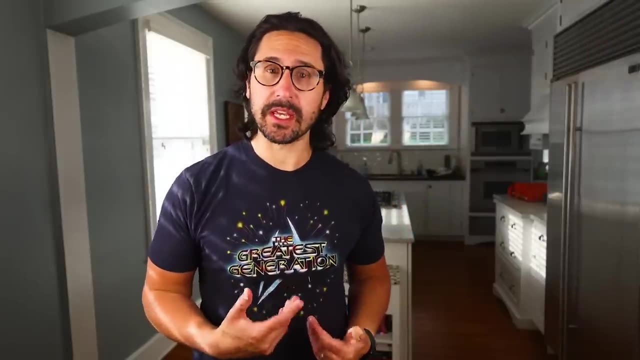 yeah, now I see what the butcher meant. The Chilean lamb tastes totally different. It didn't taste bad, mind you, but that meat had some flavor notes in it that were totally unfamiliar to me. Strong ones too. New Zealand lamb is famously mild, and I've had some domestically raised. 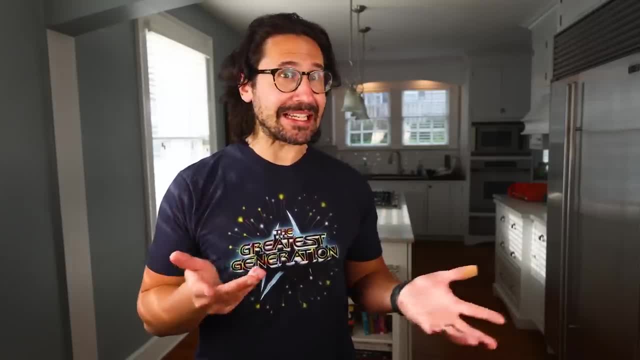 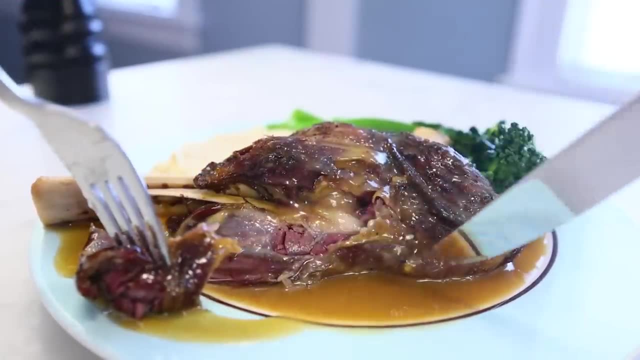 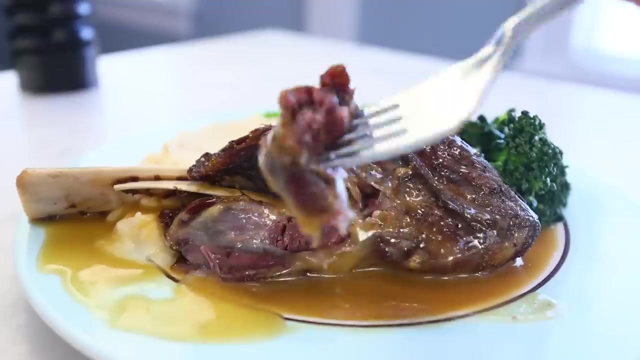 lamb from here in the United States that tasted disappointingly indistinguishable from beef, That is to say no sheepy taste at all, And so I'm really not sure I can say that lamb is my favorite meat, because that sheepy flavor is not just one thing Scientists have identified. 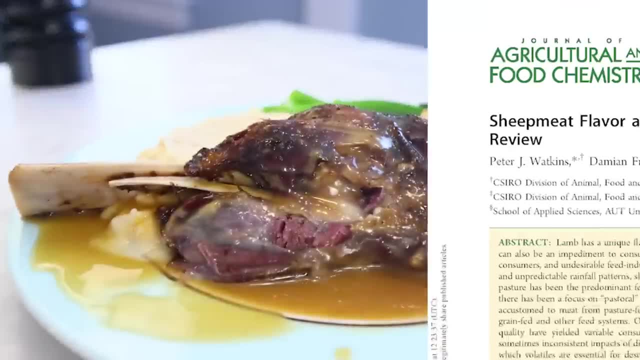 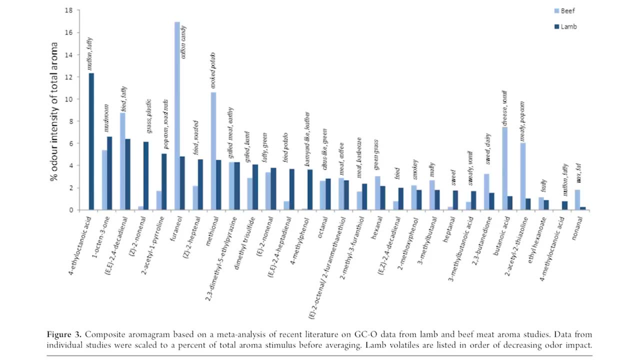 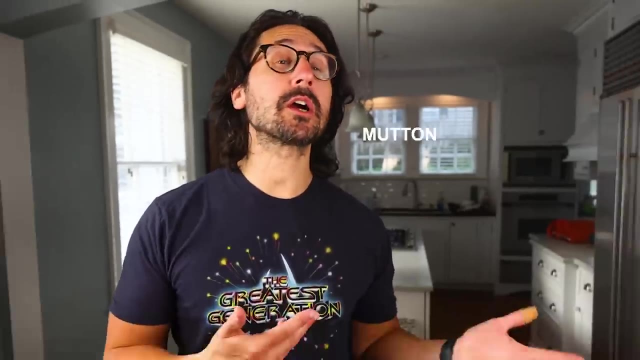 many different organic compounds that characterize sheep meat, and they vary enormously depending on the breed and the species. The meat of an adult sheep is known as mutton, and mutton is virtually unheard of here in the United States. I mean there's some recent immigrants who have brought a taste for mutton. 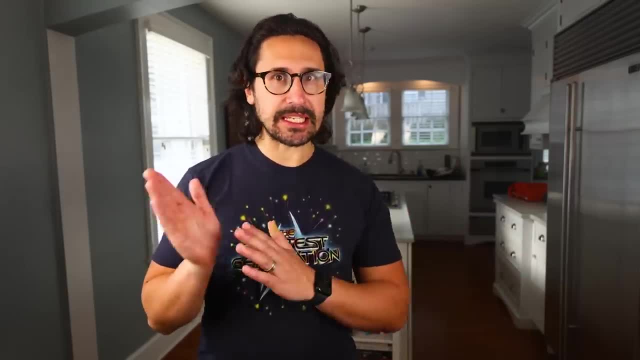 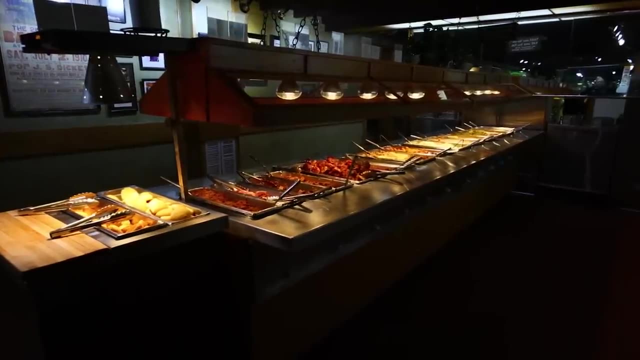 with them to this country, And so in big cities, particularly in the East, you might find some a little bit of mutton frozen in like a halal grocery. for example, Mutton is much stronger in taste than lamb And, as near as I can tell, there was only one place in the US that 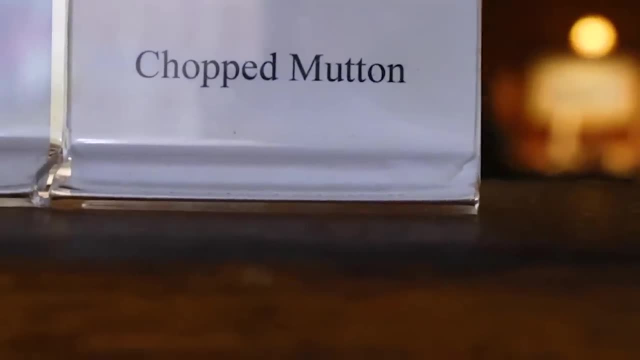 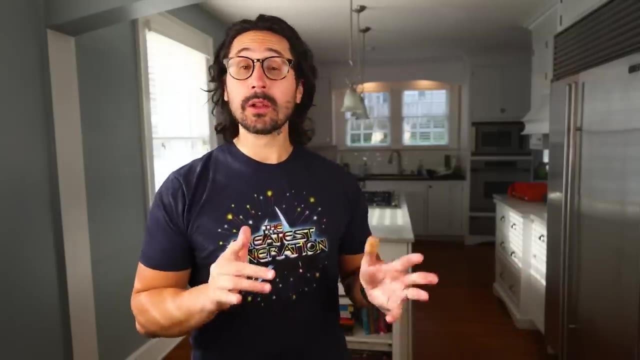 I've ever been to, and that's in the United States, where white people still eat mutton as a matter of tradition, And we will visit there. before we finish today, Before we talk about how age affects sheep meat flavor, though, let's talk about breeding. 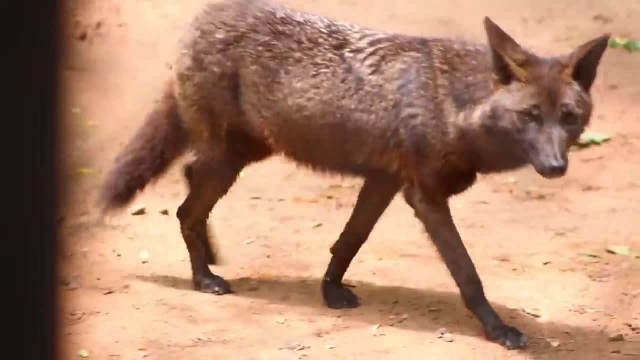 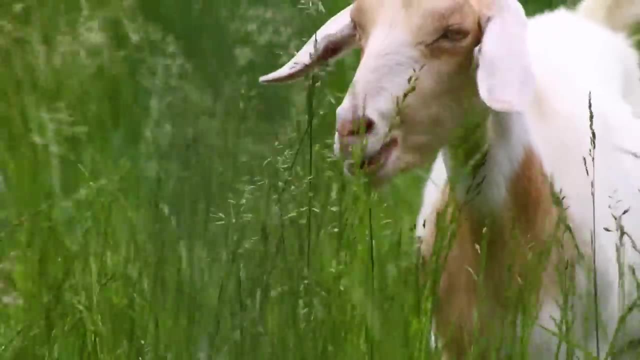 Dogs were the first animals domesticated by humans, but that was in a hunter-gatherer context. At the dawn of agriculture, about 10,000 years ago, sheep and goats were among the first animals domesticated. Goats like this guy are closely related to sheep. They taste pretty similar And indeed, 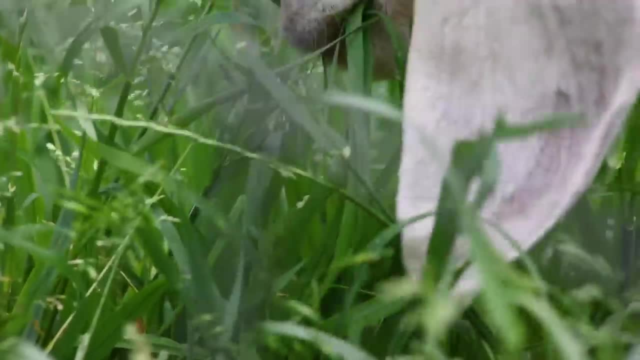 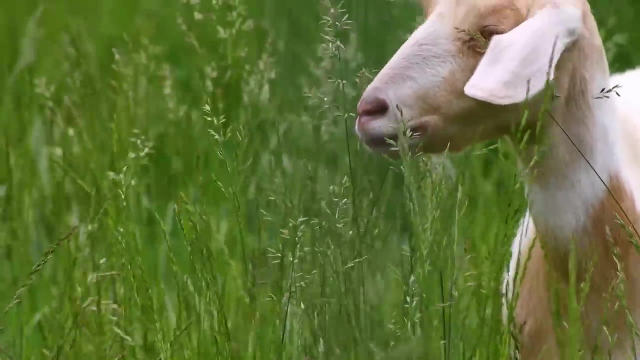 refers to goat meat in South Asian and Caribbean cuisine. Sheep and goats are incredibly hardy creatures, tough little guys, capable of thriving in a vast array of climates. This is probably one reason why there is much more genetic and flavor diversity among modern domestic. 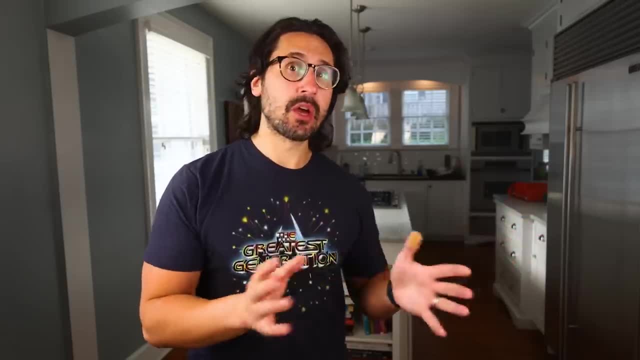 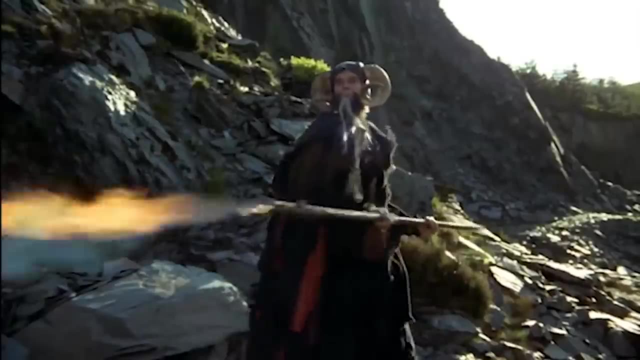 sheep than there is among cattle or pigs or chickens. The original wild ancestor of the sheep was probably — this guy is called a mouflon. Sheep and goats are a very common breed. They come from around the Caspian Sea area. But 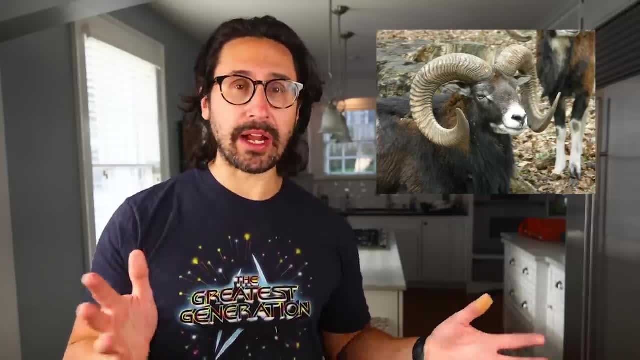 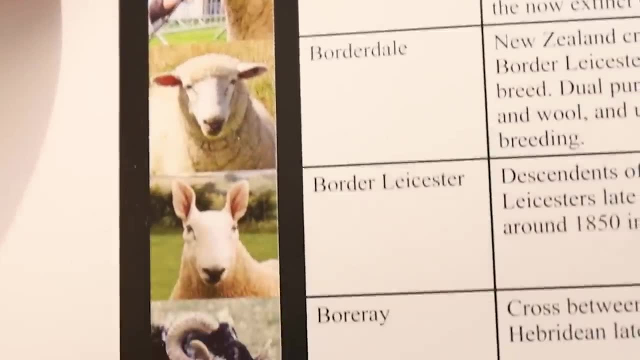 with a little bit of breeding, sheep can live just about anywhere, and so they do. Look at all these different sheep breeds — sheep with horns, sheep with no horns, white sheep, black sheep, brown sheep, sheep with long flowing wool, sheep with short curly wool. 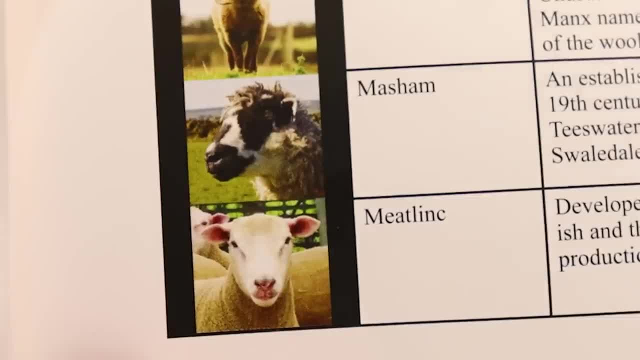 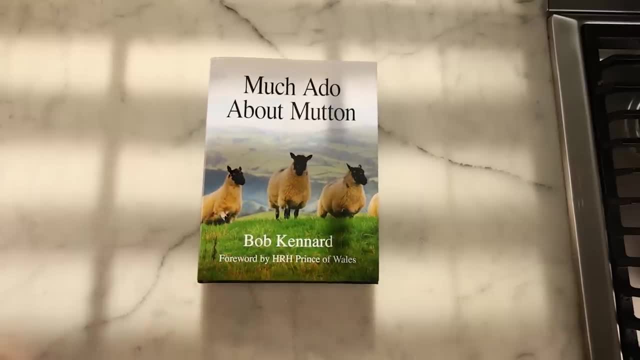 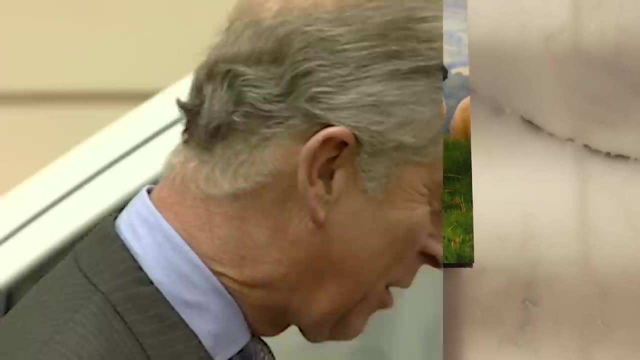 sheep with no wool at all, hair sheep suited for hot climates. So many different kinds of sheep- And most of these are just the British breeds- documented in a lovely book called Much Ado About Moulin, Much Ado About Mutton, by Bob Kennard, with a foreword by HRH Prince of We, Oh His, 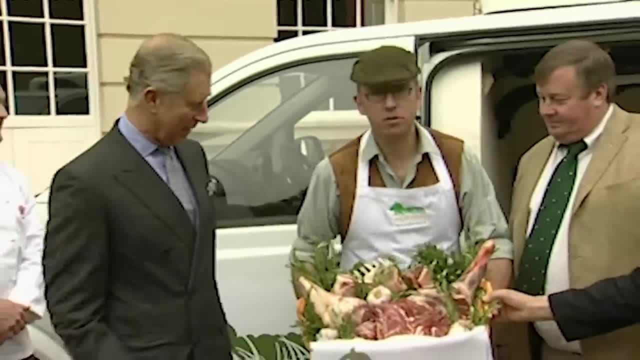 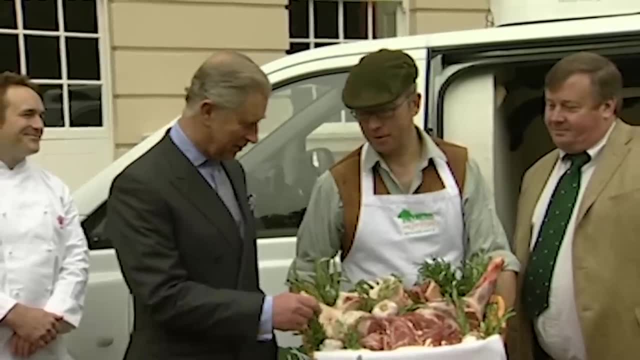 Royal Highness Prince Charles is a noted fan of mutton. It's his favorite dish. he says, Oh, and by favorite Brits, of course I mean favorite. Anyway, Charles sponsored a whole campaign some years ago called the Mutton Renaissance, trying to get Brits to. 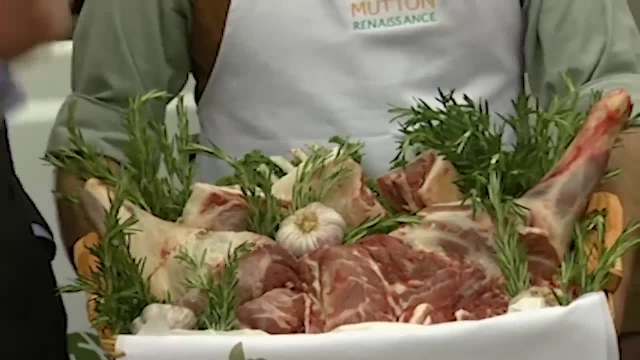 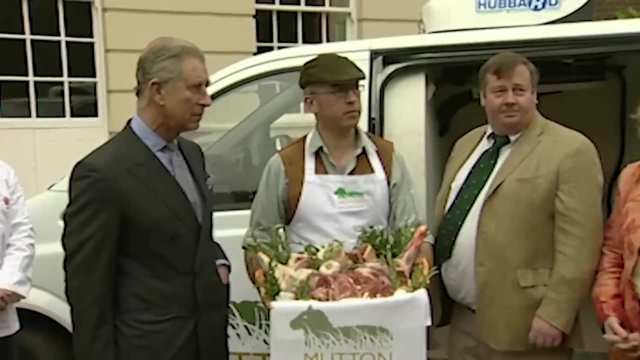 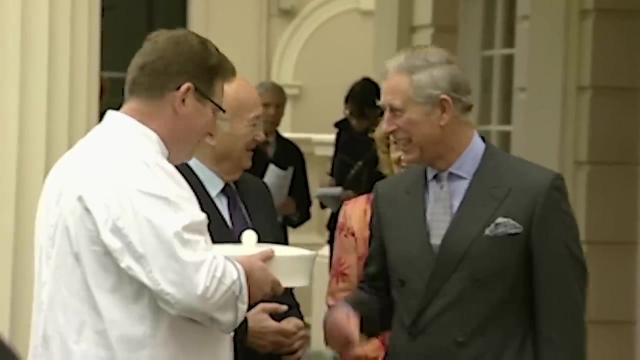 eat more mutton and help out UK farmers who often have trouble selling their older animals, For example breeding females called ewes that have reached the end of their breeding days. Brits still eat a lot of lamb- younger sheep, far more lamb than us Americans eat- but Brits eat hardly any mutton anymore, despite the fact. that they used to eat a ton of it. British sheep were originally bred and kept chiefly for wool, also a little bit for their milk and to some extent for the fertilizing power of their manure. You'd let your sheep graze on a field one year. they'd poop all over. 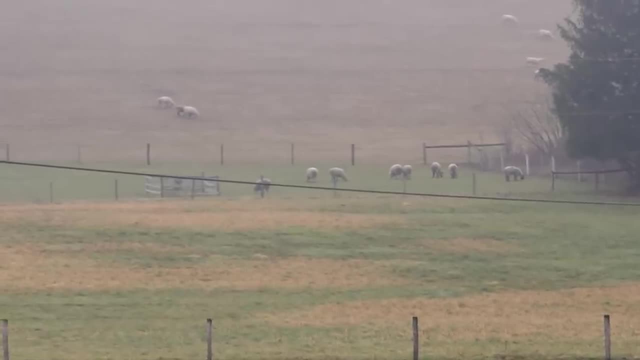 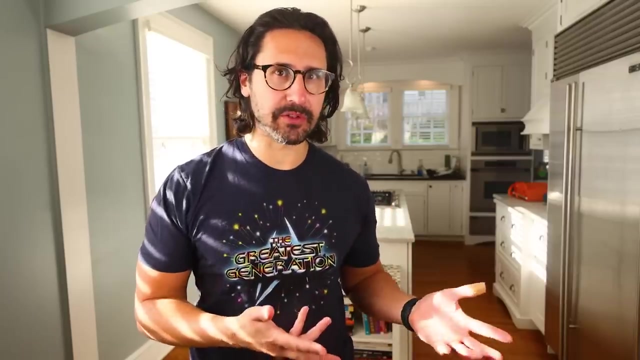 it and then the next year you'd plant grains on that same field and you would get a great crop. Another example is why the Brits kept sheep. Sheep eating has a deeper history in those parts of the world where there's a cultural and religious aversion to eating pigs- Christians in Britain ate pigs just fine. so they sheared sheep And indeed breeds developed for wool are reputed to taste pretty awful. Some of them just like far too much fat, hardly any lean at all. Some people say that they can taste the lanolin. You know, it's this waxy. 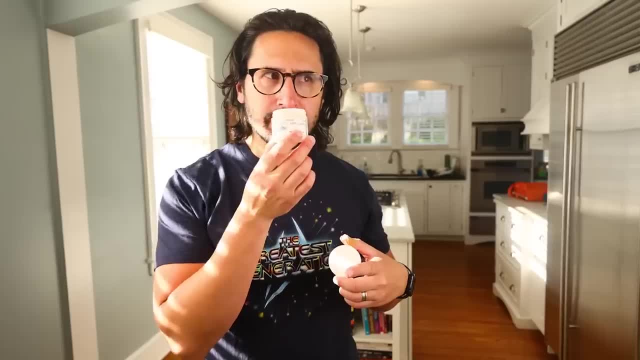 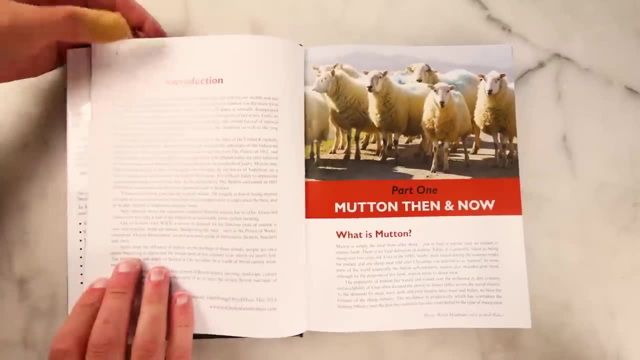 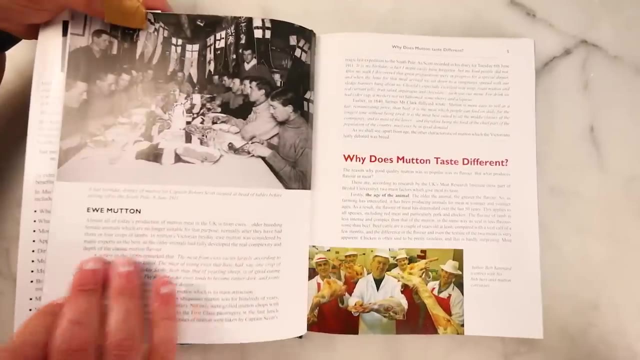 substance that's naturally found on wool. It's used in cosmetics. Yeah, I suppose I wouldn't want to have that flavor in my meat, But as Bob Kennard documents in his book here, Britain's industrial revolution created a huge new demand for food in the cities. People working in factories needed to be fed, and 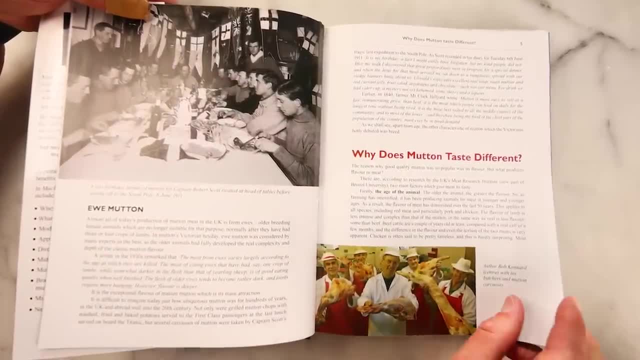 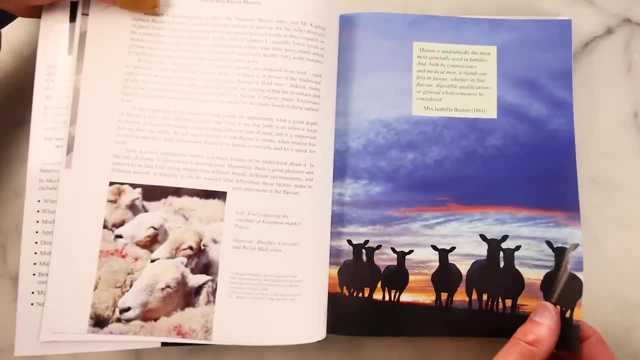 they were often weaving textiles out of newly imported cotton rather than wool, because consumers generally prefer cotton when they have a choice, and so the obvious choice was to eat the sheep. The meat of adult sheep is cheaper because there is more of it compared to a little lamb than sheep. But the meat of adult sheep is cheaper because there is more of it compared to a little lamb than sheep. 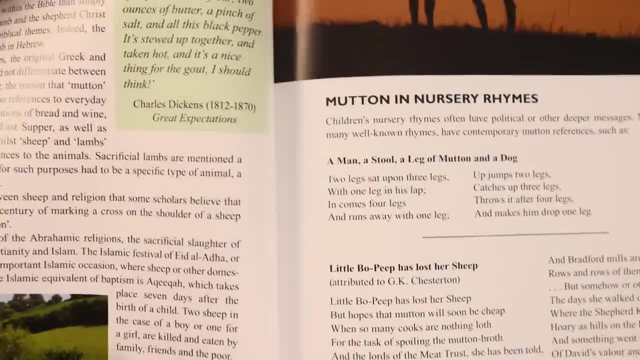 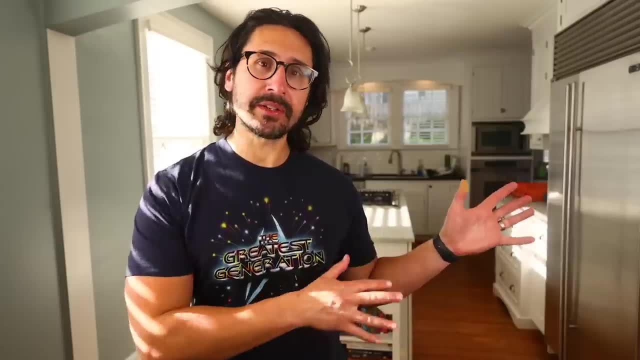 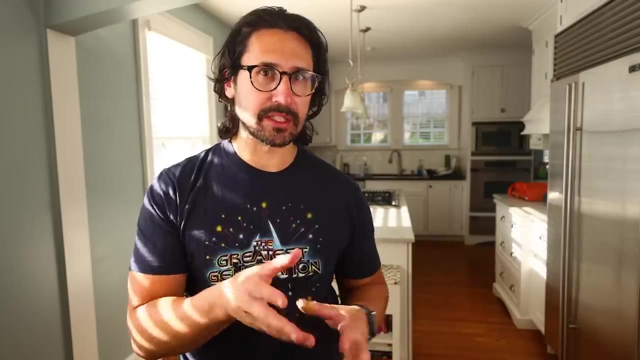 And thus references to mutton, permeate, Victorian-era culture, Nursery rhymes, literature, righteous facial hair. And then shepherds in Britain and the colonies started to develop new breeds of sheep specifically for meat — breeds that tasted way better and had a lot more lean relative to the fat. 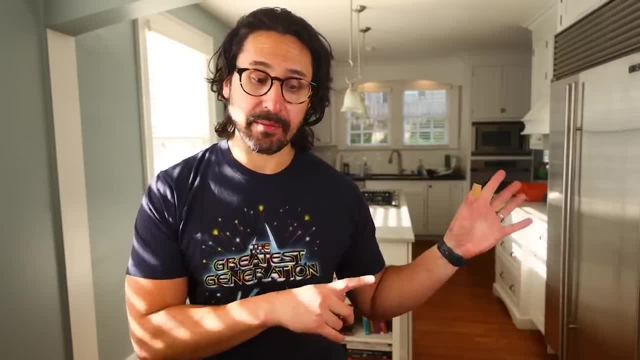 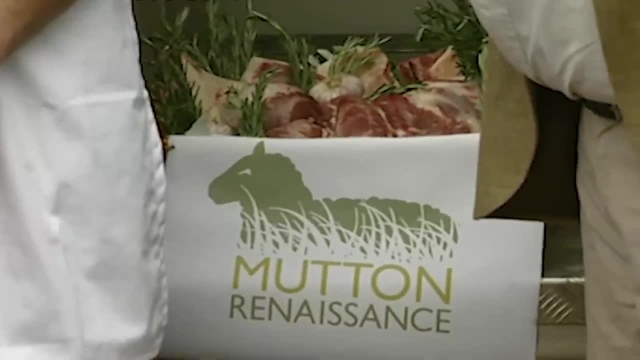 Most of the strong flavors in sheep come from the fat. We'll get back to that, But the problem remained that mutton adult sheep meat is extremely tough and has to be cooked low and slow. Indeed, when I cooked these lamb shanks — that I suspect might have been from slightly older 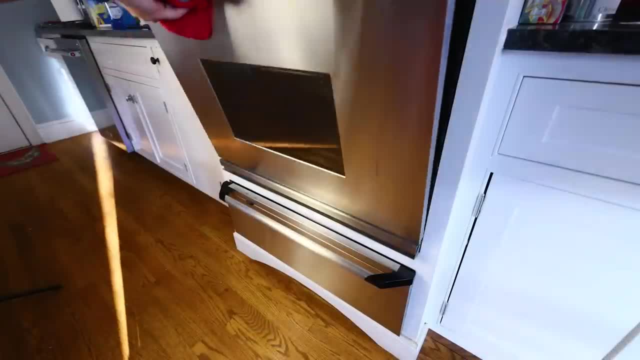 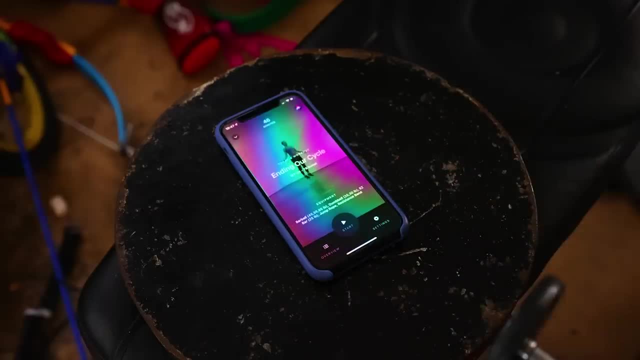 animals, maybe hoggets — they took like half a day in a low oven. So I said, screw it, I'm gonna go and do my workout with the sponsor of this video, Future. Future is a new fitness app that pairs you with a real, highly qualified coach like my man, Jose. 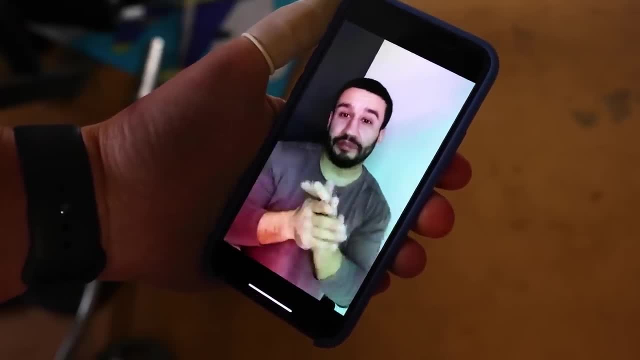 Adam, my man's a-jumpin' in this, Say hello, say good morning. Jose, structures custom workouts for me based on my goals and what equipment I have available, and then I just follow them right off my phone. Future sent me a link to my YouTube channel. 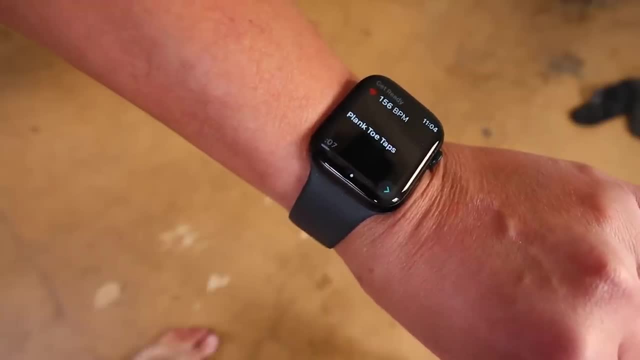 and it's a great way to get in touch with people who are interested in my work. and it's a great way to get in touch with people who are interested in my work. Future sent me a watch that tracks my vitals and tells Jose exactly what I'm doing or not doing. 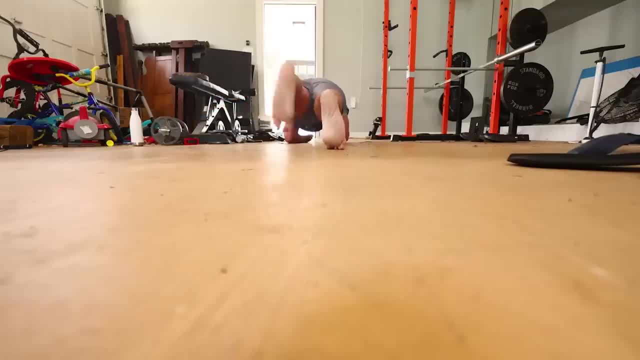 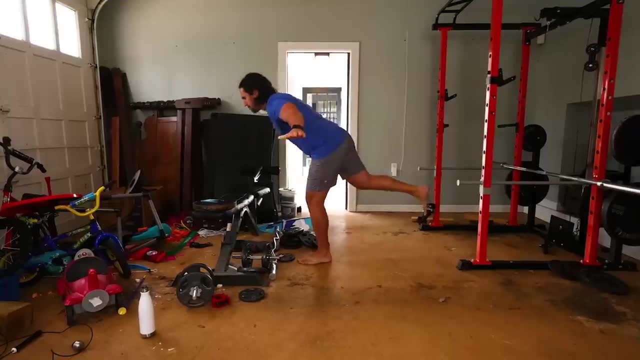 so I've got personal accountability. It's great motivation and I have seen some remarkable results in just the last month or so. In addition to my normal barbell stuff, Jose has me doing all these plain old bodyweight exercises that I don't want to do because I'm embarrassed. 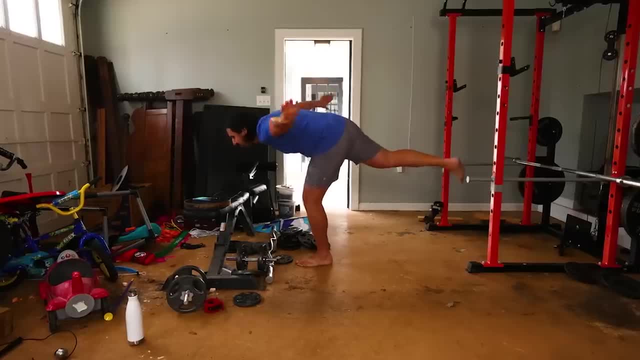 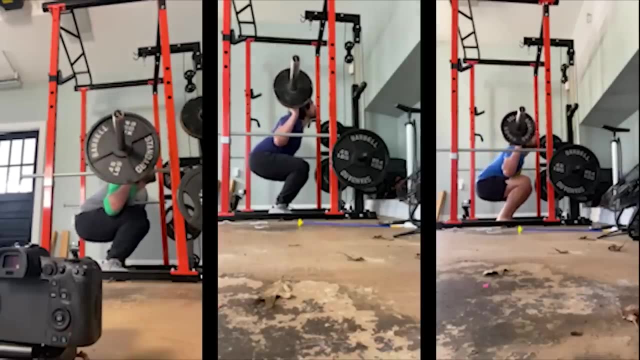 by how awful I am at them, but I can do them in the privacy of my garage and they are fixing all of these dysfunctions. I had Jose compiled three weeks of my progress on the squat and look at how much better my form is on the right. That's mostly from these bodyweight. 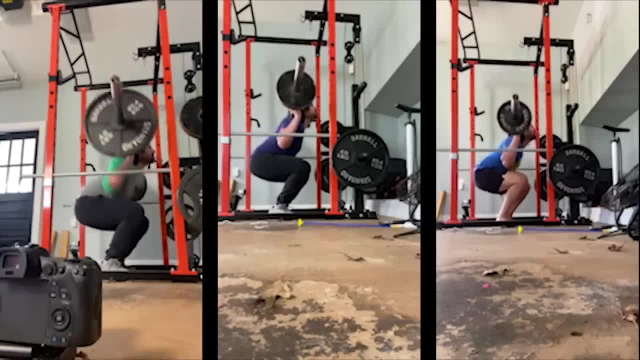 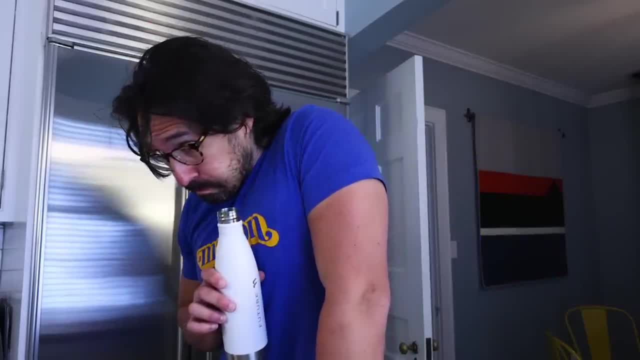 exercises strengthening my core and my posterior chain. My wife says I suddenly look taller, probably because my posture is better. You don't have to have any of the equipment that I have. Future will craft workouts for you, no matter what your situation is. Use my link. 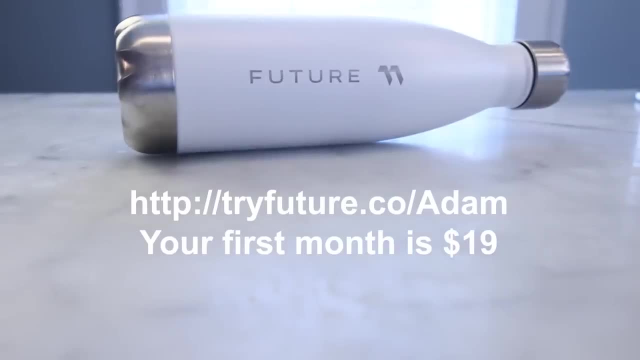 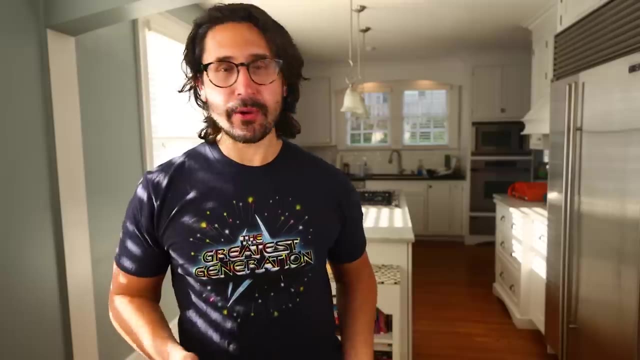 in the description and you can try a month of Future for just $19.. Try futureco, slash Adam to get your first month for 19 bucks. That's in the description. Thank you, Future. But anyway, we were talking about the past. 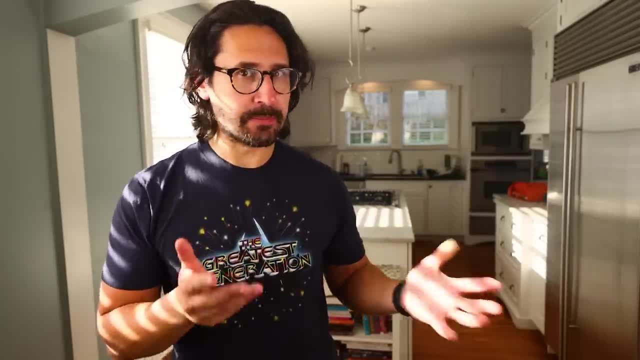 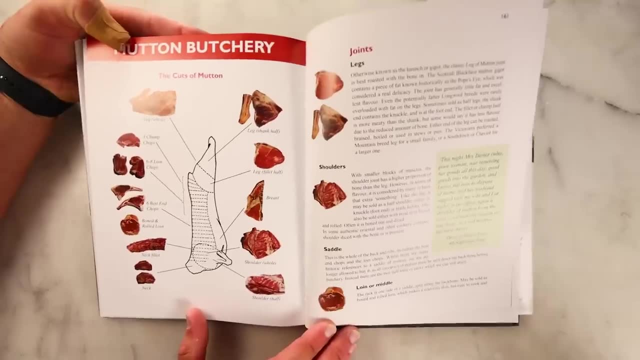 The days in Britain when mutton was king. Good mutton is great, but it's very strong and very tough. You can get steak-like cuts from a mature sheep but almost nobody cooks them like steaks grilled to medium rare. Mutton is just too tough for fast cooking. 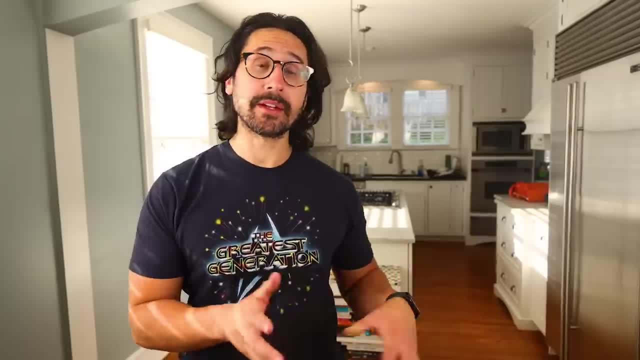 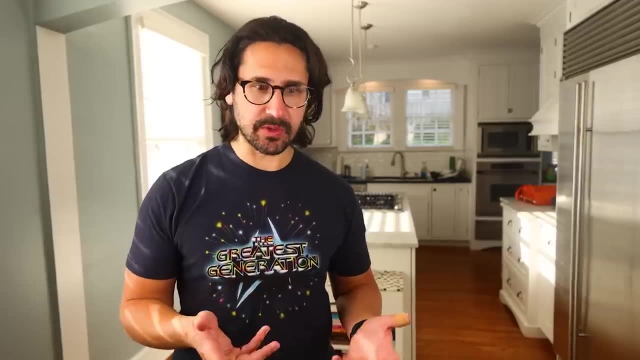 You have to mince it or slow cook it for hours. A lamb, on the other hand, is tender, so it's been a delicacy since biblical times, right? It's a very inefficient thing to produce, which is why it's still expensive to this. 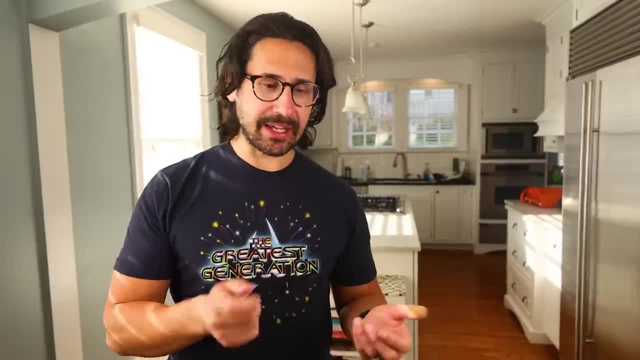 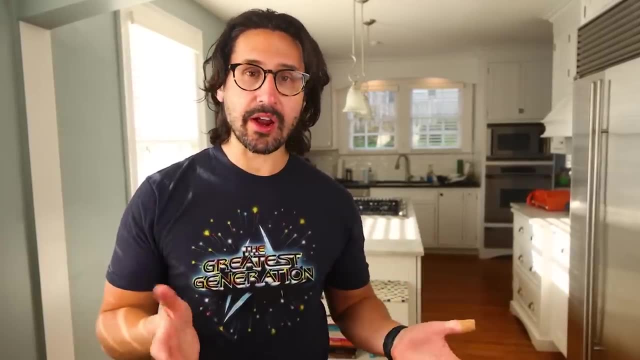 day, because lambs are small and also you have not yet gotten several crops of wool out of it before you slaughter it, So it's very resource intensive, which is why it's historically regarded as this special treat, this special thing for holiday feasts, for 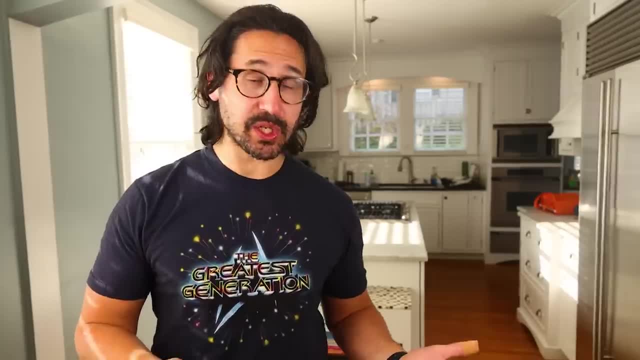 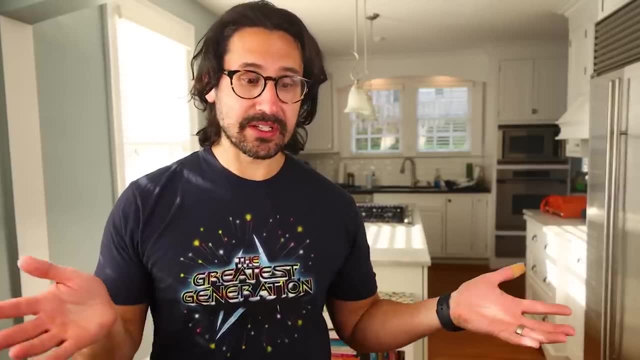 example. But with the rise of industrialization and globalization, all kinds of previously special treats have become everyday fare for us right? And so it is the case with lamb. When most people in the wealthy West eat sheep, nowadays it's lamb. 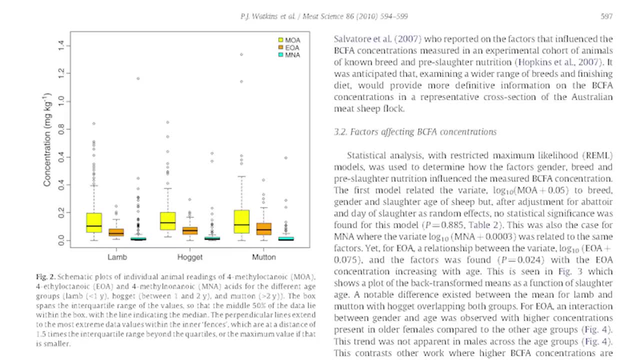 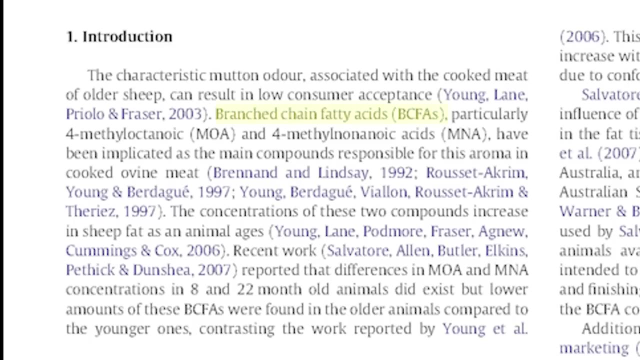 And lots of research verifies that lamb has less of those strong flavor compounds we associate with sheepy taste. What are those compounds? Chiefly they are branched chain fatty acids. This is one of the early studies on the topic, a 1975 paper by New Zealand government scientists. 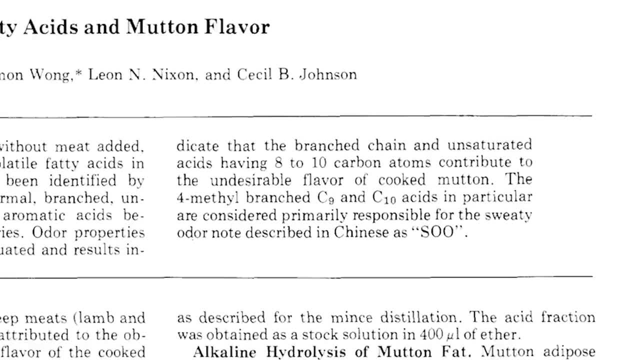 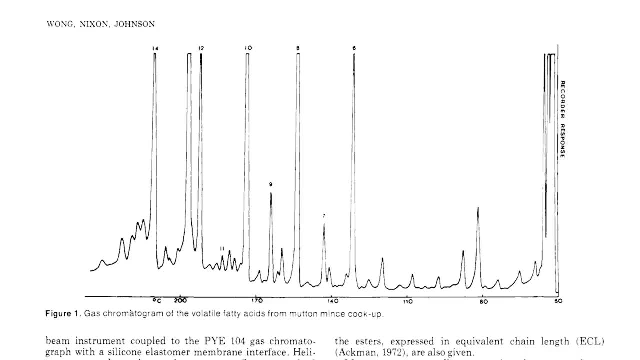 who were basically trying to figure out how to sell meat to Asia. They mention a Chinese word, sou, that describes an undesirably sweaty aroma of sheep, And so they used distillation and gas chromatography and such to try to isolate the SO compounds that Chinese consumers 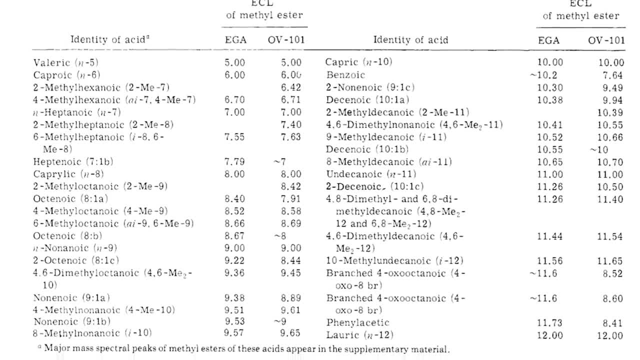 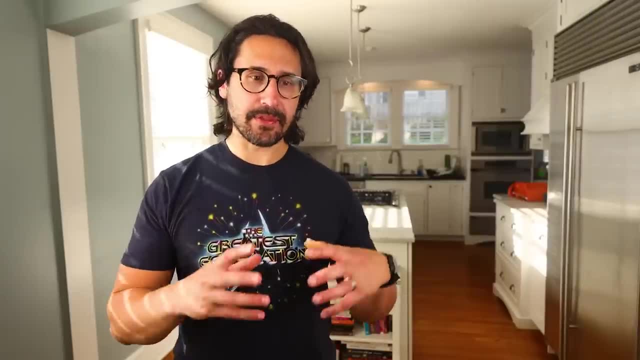 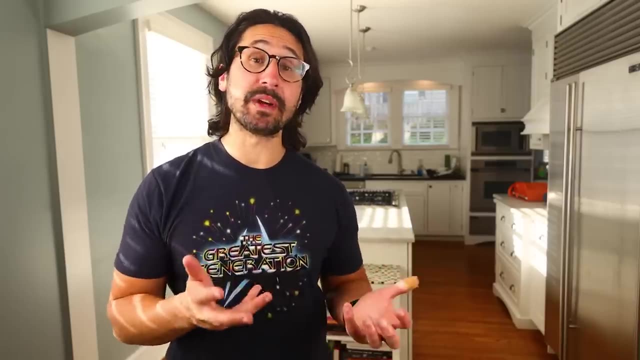 apparently hate, which turned out to be 4-methyloctonic and 4-methylnanonic acids — volatile medium-chain fatty acids. It is thought by scientists that these special-smelling fatty acids are created via metabolic pathways in the animal associated with rumination. 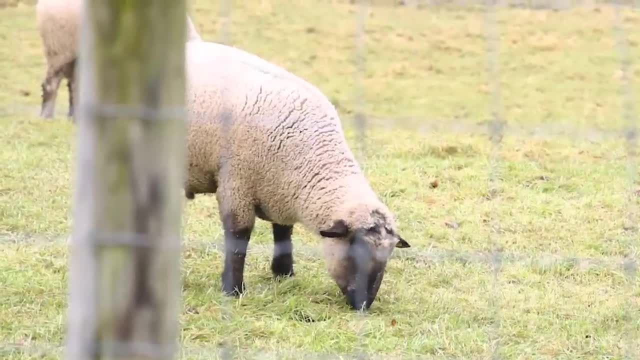 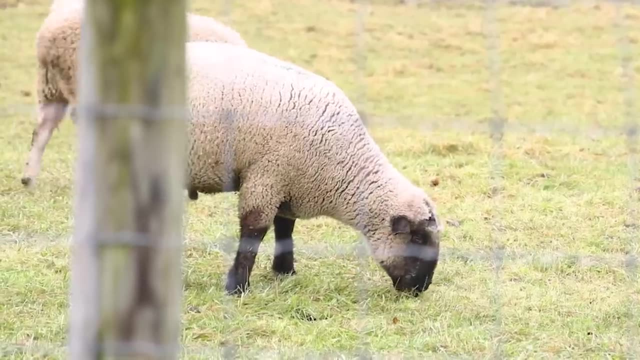 Sheep eat grass, but not directly. The indigestible cellulose in grass must first be fermented by bacteria living in the sheep's multi-chambered stomach — its rumen And all kinds of interesting flavor compounds result from the interaction of the grass and the bacteria and the sheep. 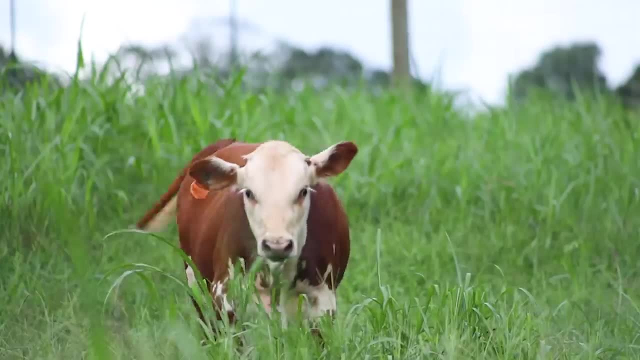 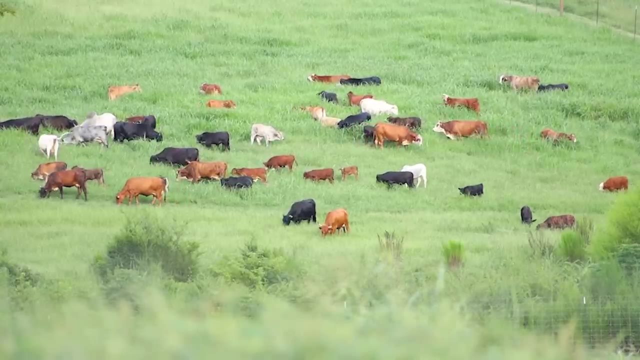 such as branched-chain fatty acids. Grass-fed beef often has BCFAs as well, and sometimes you can taste them in the meat. When I lived in Georgia, I got grass-fed beef from this place called Rocking Chair Ranch that I heartily recommend. This beef had what I perceived. 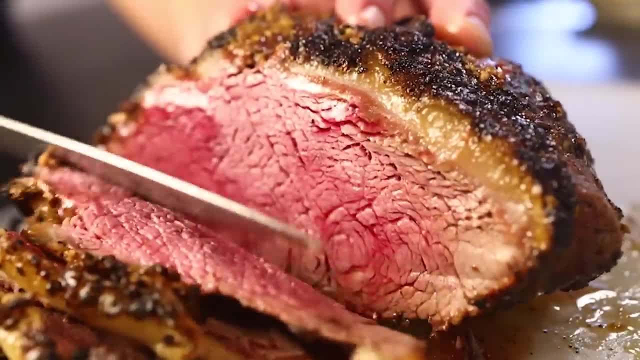 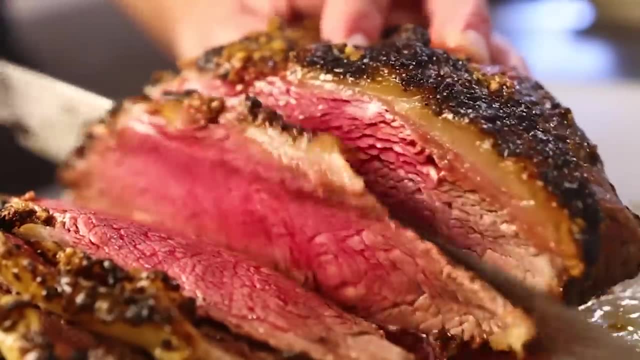 as a pronounced lamb flavor in the fattier cuts. That could have also come from this orange peel they used in supplemental feed. Do the cattle eat orange oil there? Regardless, that beef tasted delicious — Rocking Chair Ranch. But mainstream beef is generally at least finished on grain, That is, it eats grain. 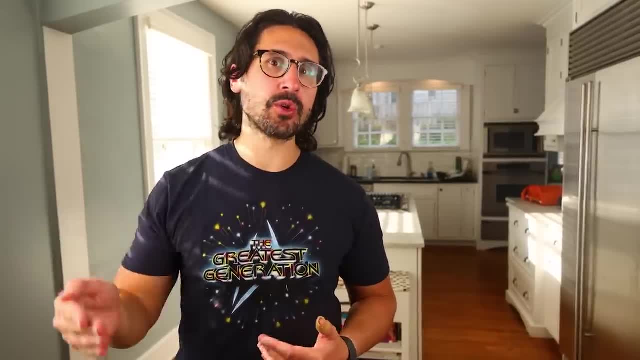 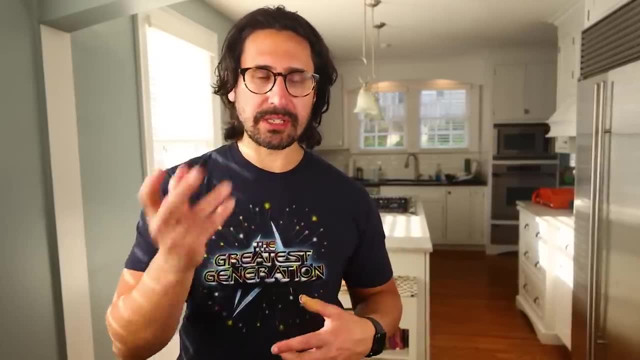 almost exclusively — or exclusively — in the months leading up to its slaughter. They do this to fatten the beef, but it also seems to have this effect of diluting those strong-smelling fatty acids that are in the meat, if they were there at all in the first place, And it sort of standardizes. the meat makes it less smelly, And sheep are sometimes grainy, And sheep are sometimes grain-finished as well, sometimes to the point where they barely even taste like sheep. That's a criticism I have of some American lamb, though certainly. 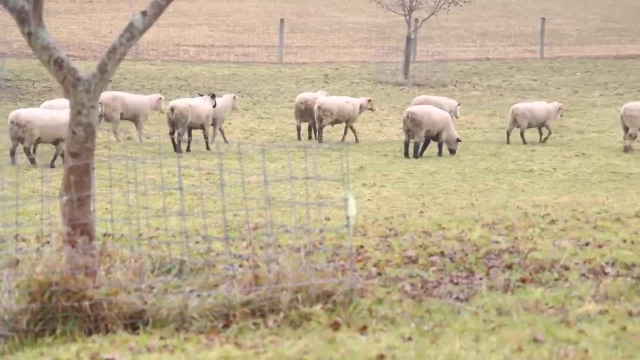 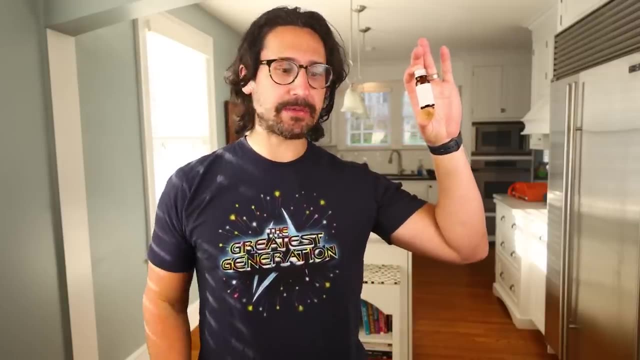 there is some amazing American lamb too. What exactly do these characteristically sheepy fatty acids smell like? Well, I can tell you, because I happen to have some in a bottle, courtesy of a bloke named Harry Sherwood. Harry is a perfumer in the UK who is also 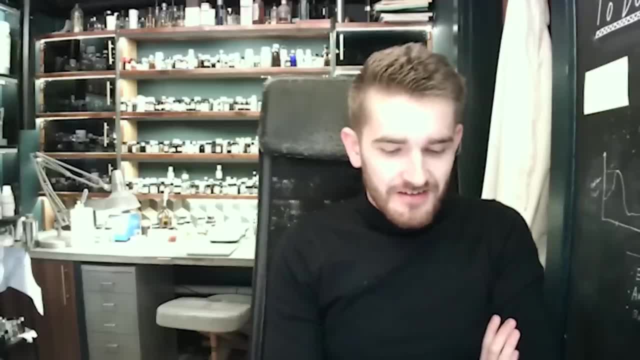 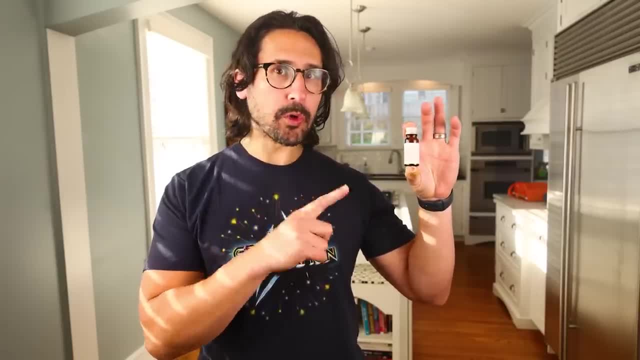 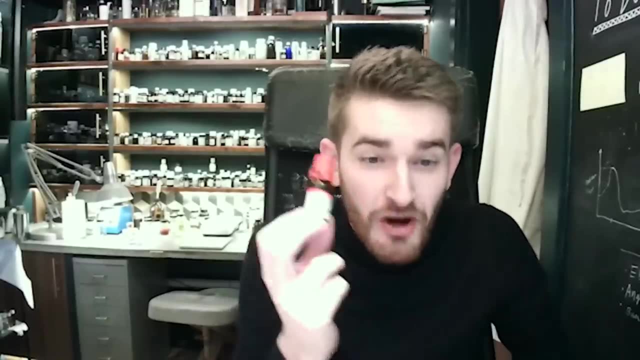 a lot, That's a lot, That's a lot. And it's made of bactonic acid. This stuff is known for its particularly low odor threshold: Humans can detect it at less than two parts per billion. I've got a neat here, so I'm going to just — I don't even have to open this And I. 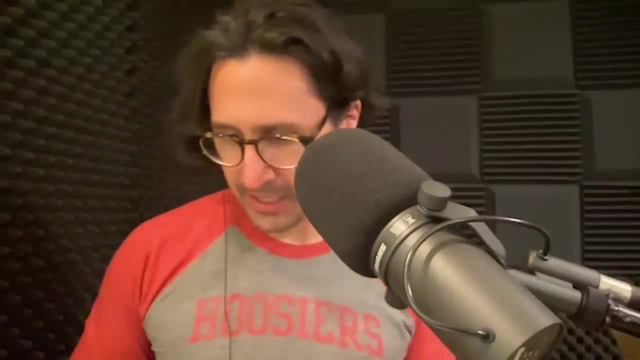 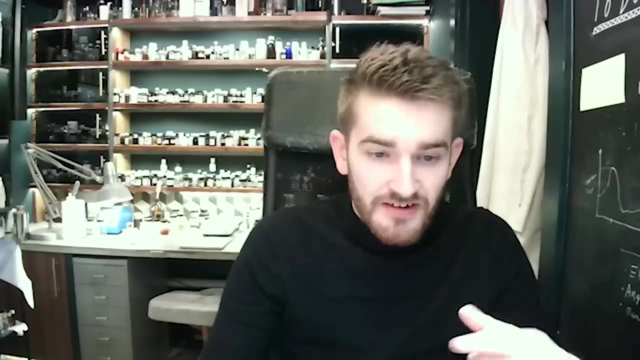 get it. So when you say yours is neat, does that mean mine is diluted? Yours is diluted to 1%, which is more than enough, given that it occurs at parts-per-million in the meat you eat. So this is a good dose. Mine is, then, 180 times stronger than that. 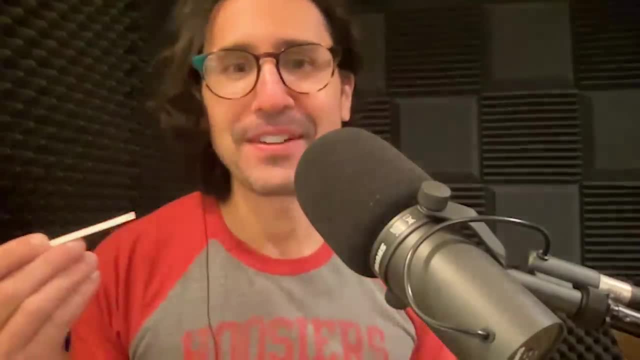 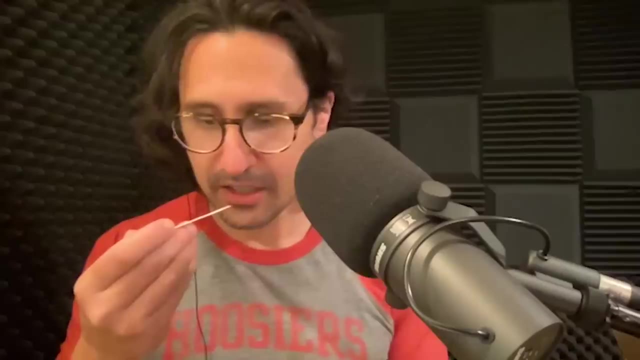 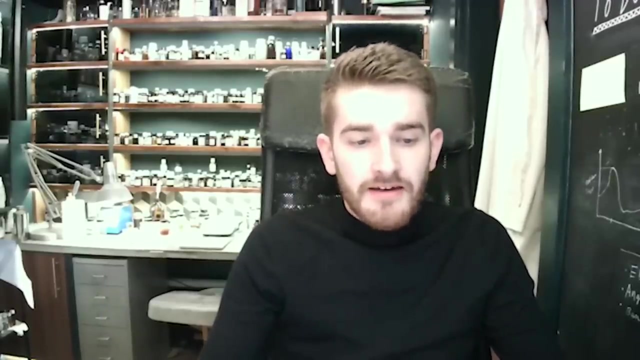 Whoa Yep, It's sheep. It's sheep, It's wool, It's all those things, But do you get the kind of unwashed hair aspect as well? Yes, I do. It's one of the strongest fatty acid components of meat And, according to the research from 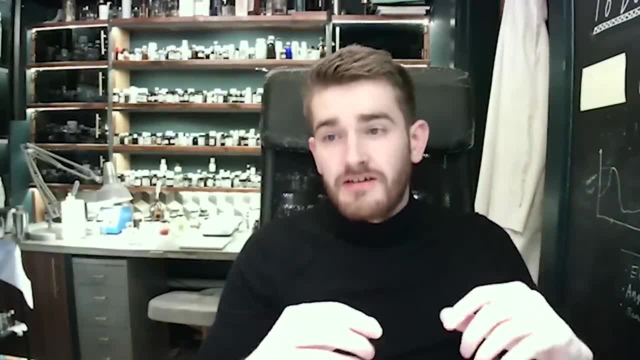 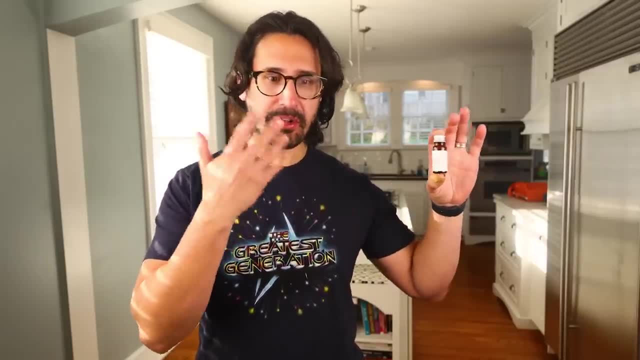 what we know together as a lamb ages, the concentration of this increases in the meat, And sheep can have varying proportions of these different smell compounds depending on how they were raised, their sex, how old they were when they were slaughtered. what 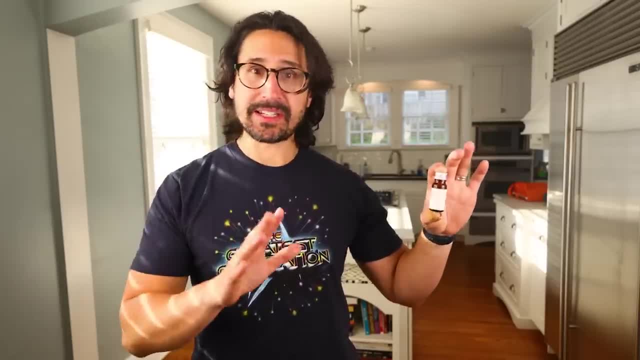 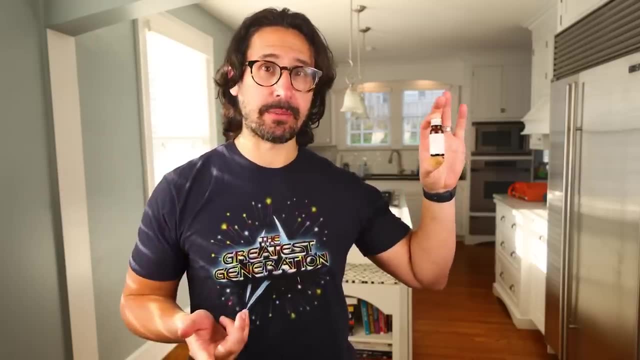 breed they were all that kind of stuff — the forage they ate. Plus, there's other things in sheep meat that make it taste sheepy, not just the medium-chain fatty acids we've been talking about. This paper mentions the use of linoleic acid as a feed supplement in the lamb industry. 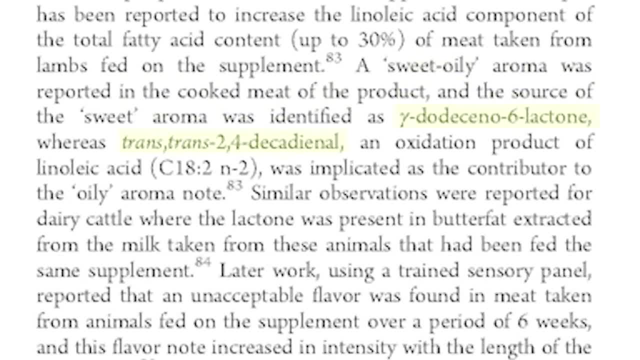 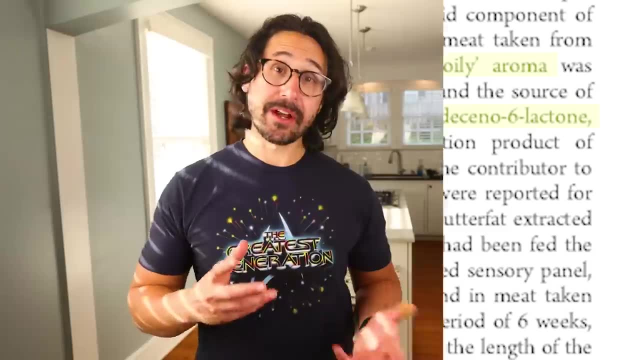 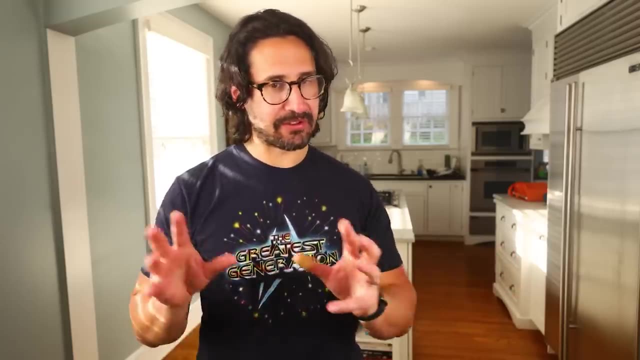 That's a polyunsaturated fat prone to oxidation. Here's a resulting oxidation product found in lamb meat that consumers identified as a sweet oily aroma. Of course, another name for lipid oxidation is rancidity. Lipid oxidation creates lots of flavors that we like in some contexts and we find very unappealing in others. It sort 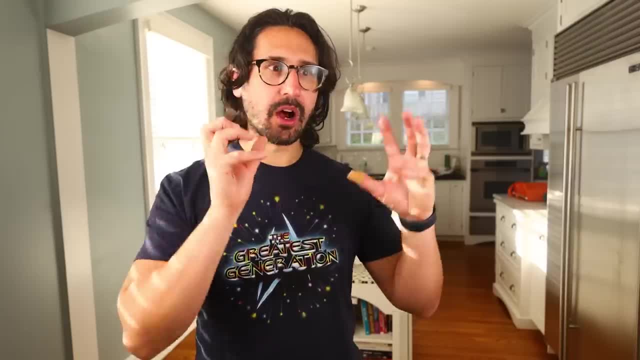 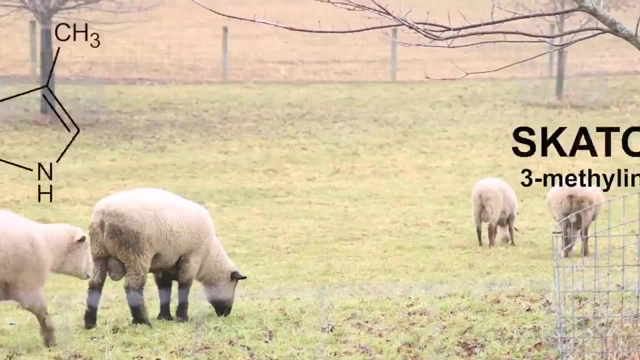 of depends on the concentration and, potentially, what other smells are around it, as is the case with another compound that is found in lamb meat sometimes and that is called scathol. Scathol is thusly named because it is one of the smells of poop. 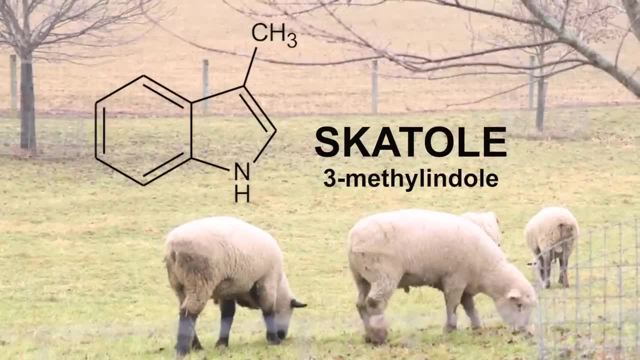 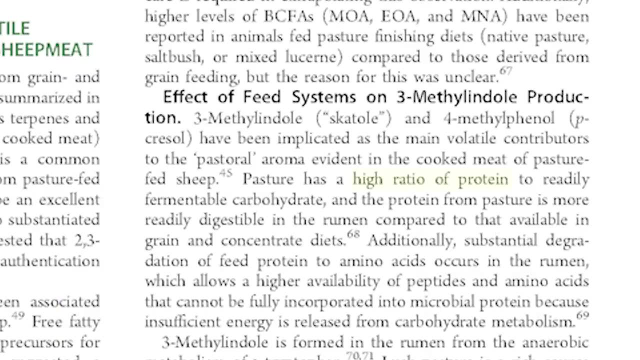 Scat 3-methyl lindol is created by the digestion of the amino acid tryptophan, and the research indicates it is particularly present in sheep that have gotten either naturally high-protein forage or protein-supplemented feed. 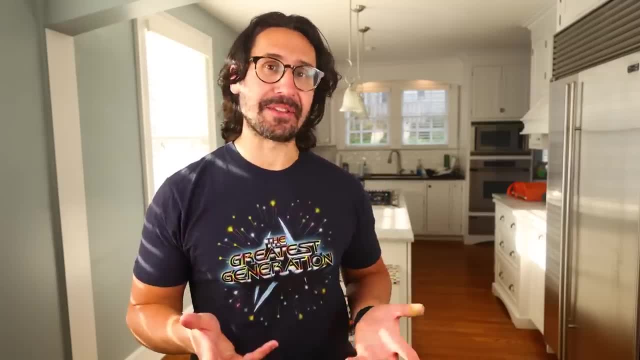 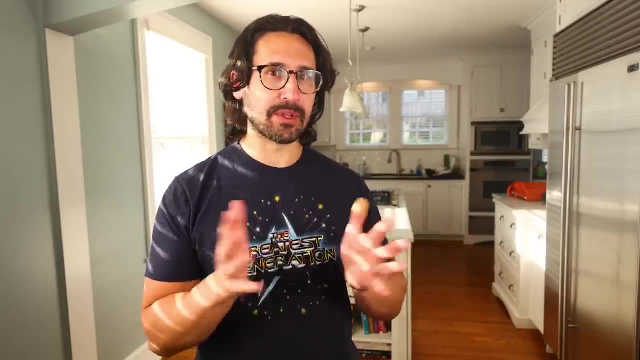 Now the weird thing is is that people have been found to actually like the smell of scathol and related lindols. as long as they're in very low concentration or if they're in combination with other certain smells, as in the case of lots of flowers, These smells are very 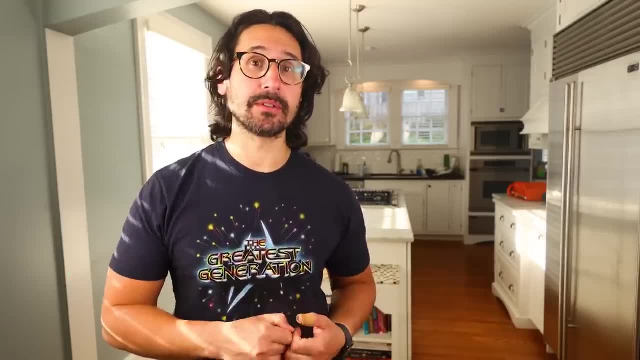 very common in sheep meat. They're very, very common in sheep meat. They're very, very, very common in sheep meat. These smells are in jasmine, for example. They've done brain studies now and they give people jasmine, a jasmine accord with, and 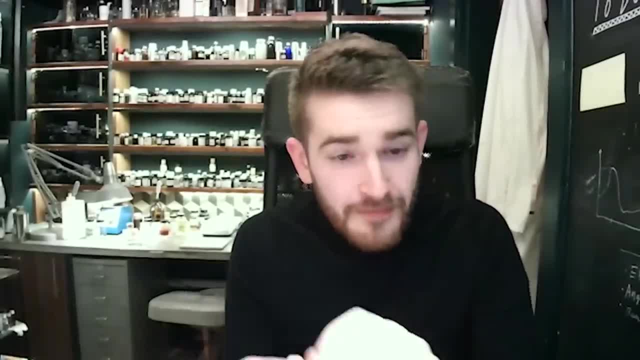 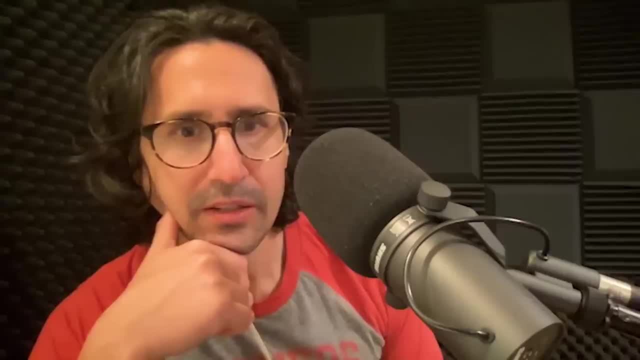 without this foul-smelling component and people prefer it and their brains light up more in their pleasure centres if it has the foul component in it, which is very interesting because you'd think, oh, humans just prefer the sweet, dainty one. But of course no. we want the real stuff, and what this molecule signals to our brain is this is a real thing. real things have bad bits in them. Real fruits have overripe components in them. Real meats have a slight 4-ethyl-oxanoic acid lamb component in them, And sheep meat has some noticeable. scathole in it as well. depending on how the sheep was raised, what it ate, all that kind of stuff And all of these kind of weird smells tend to get stronger in the animal as it ages. hence why mutton is stronger than lamb. hence why Americans don't really eat mutton anymore. or really ever. It's just too strong and we tend to like food that doesn't taste like anything, at least white Americans. Consumption of any sheep meat is just tiny in the United States, even lamb these days, which is another reason why it's so expensive. It's rare. 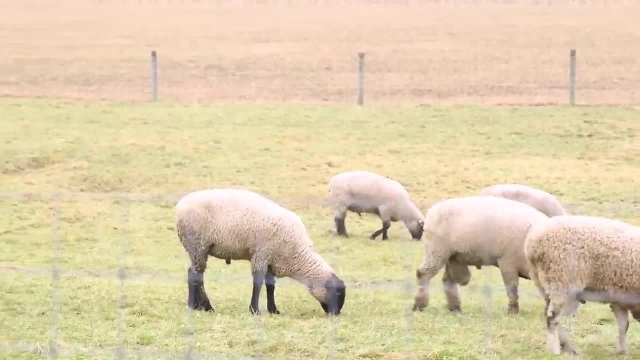 This is all due in part to historical factors. We can talk more another day about the range wars in the old American West, wars between California and the United States, wars between California and the United States. They started снова on stuff like animal herders, where they'd be. 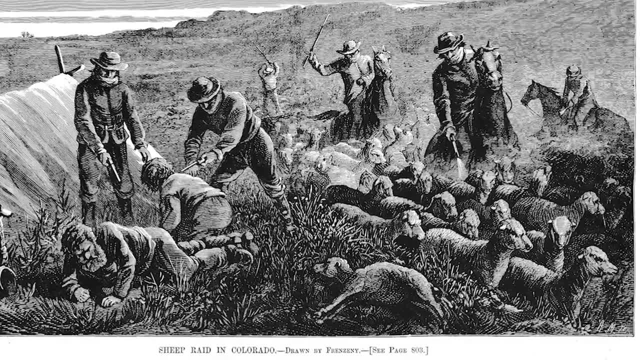 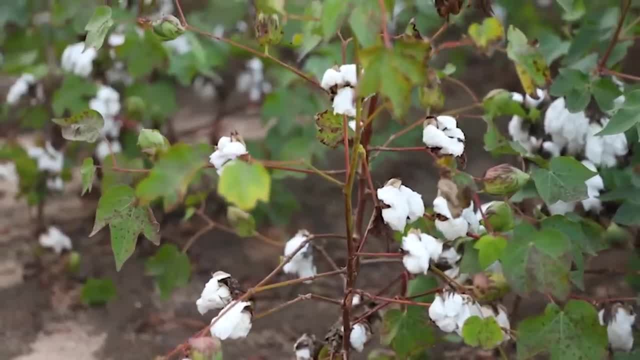 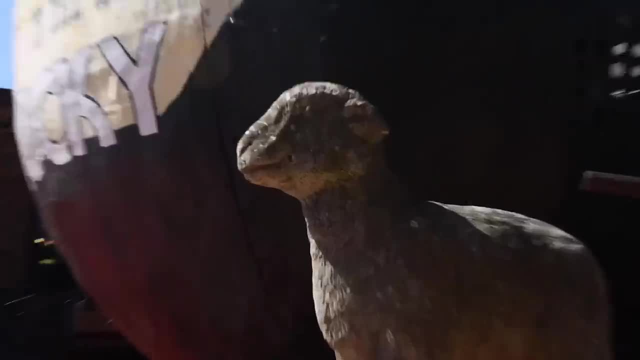 able to hunt sheepand, start some kind ofYU, And you think about it this way: this was always a sort of learning curve for sheep meat from the early", But there is one place where sheep meat reigns supreme — mutton, no less. 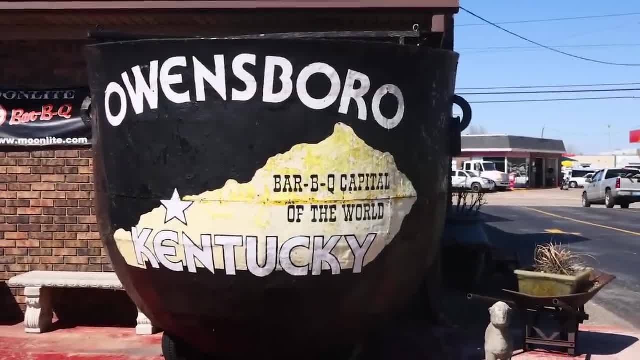 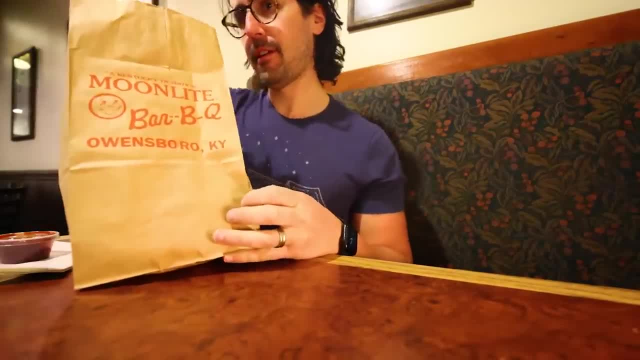 adult sheep — and that is Western Kentucky. This is Moonlight Barbecue南歌 음식& This is Moonlight Barbecue& in Owensboro Kentucky. For some reason, mutton evolved as the go-to meat for barbecue around. 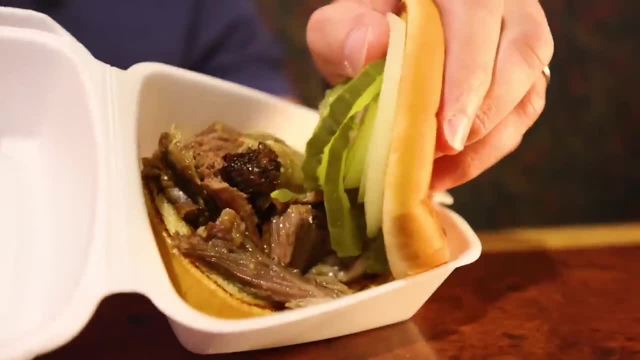 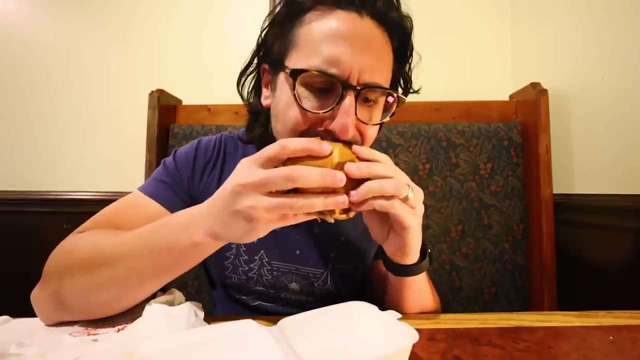 Owensboro. Nobody here knows why They speculate. it's a practice descended from Welsh settlers in this area. They definitely love their sheep and whales. Barbecue, in the American context of course, refers to tough, fatty meat that has been smoked for many hours, until very 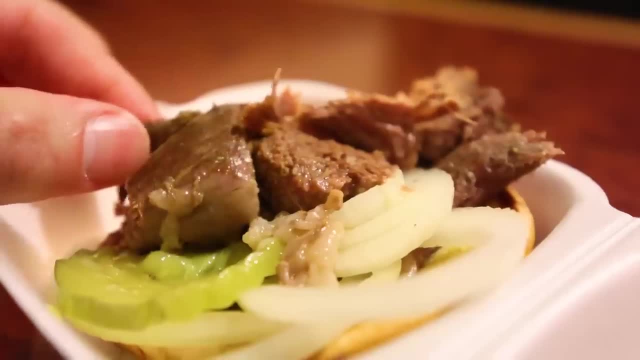 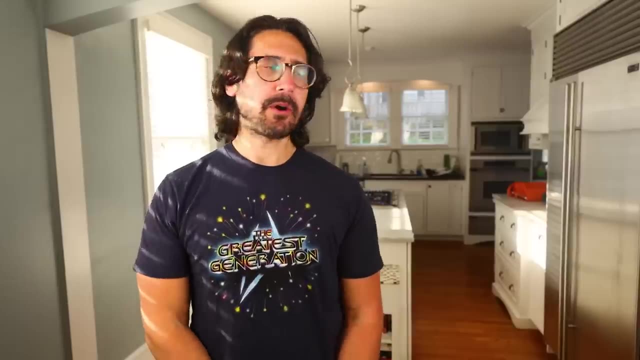 soft And indeed that is a delicious treatment of mutton. The smoke really balances all the other strong flavors, So maybe sheep is my favorite meat. I suppose it depends on the sheep. 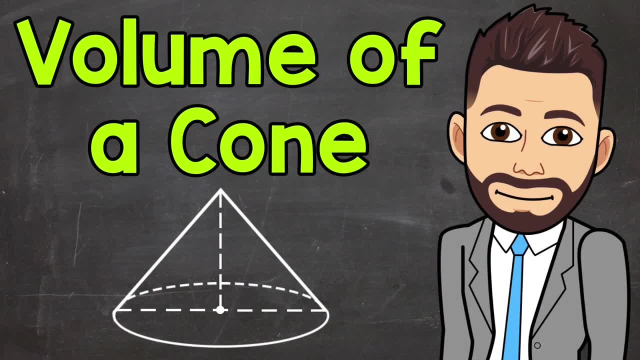 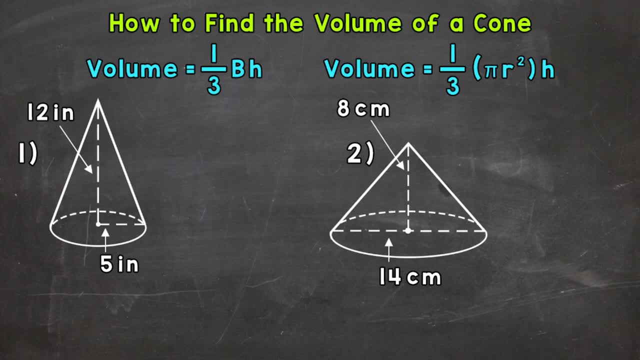 Welcome to Math with Mr J. In this video I'm going to cover how to find the volume of a cone, And remember: volume is the amount of space that a 3D figure or object takes up. Now, when it comes to cones, we can use the formula one-third times the area of the base times the height. That's the.